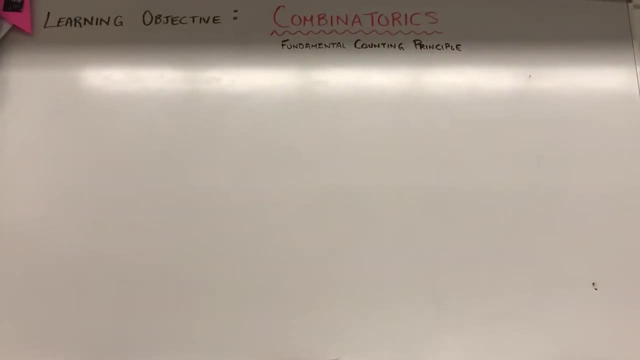 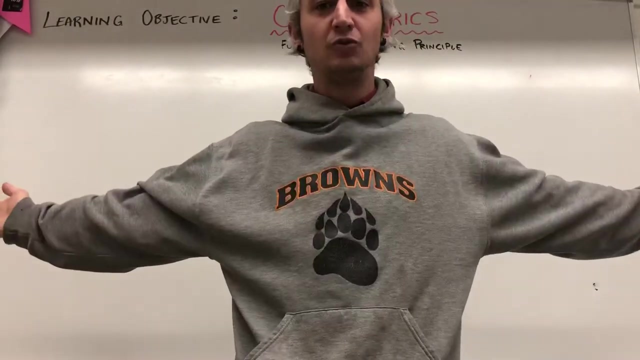 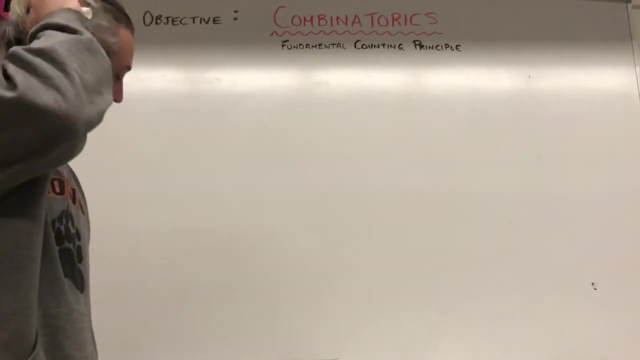 Okay, Good afternoon From the 403 to the HAZ. Mr Nelson here, Pre-Cal 12.. Hallelujah, We're moving on. We, uh, you guys should be finishing up trig Trig 1,, 2, and 3 now. And now we're moving into combinatorics. 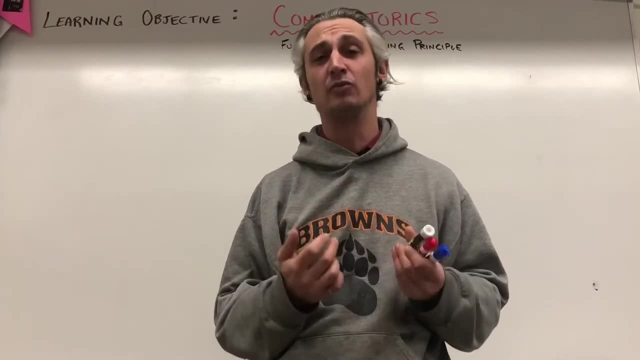 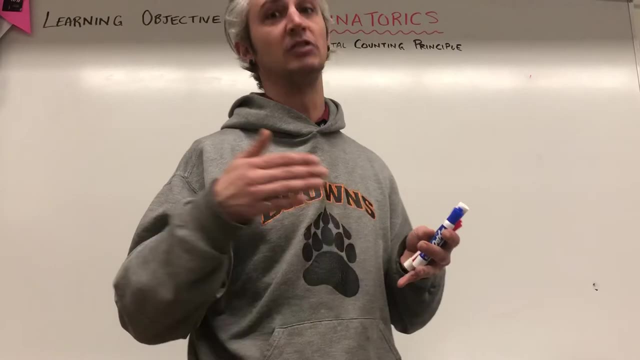 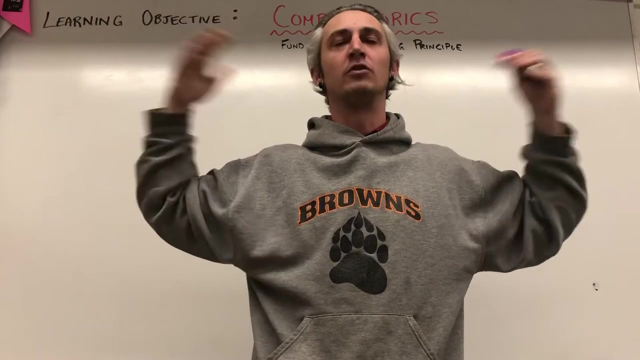 which I like because I think it has a lot of real-world applications. Combinatorics is essentially the cousin of probability and of probabilities related to statistics. So all three of these kind of make a super, a super unit. but we're only going to talk about combinatorics in uh, in Pre-Cal 12.. 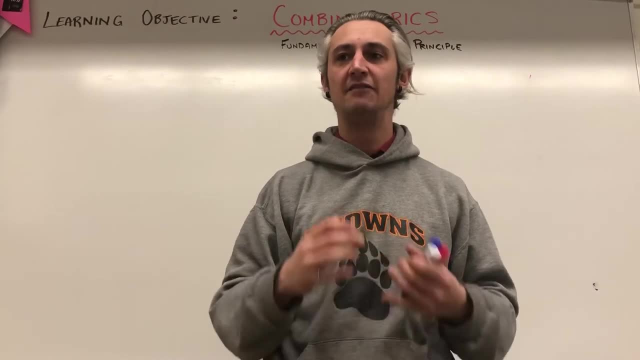 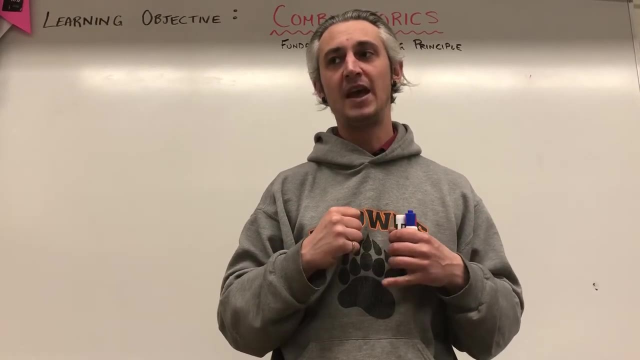 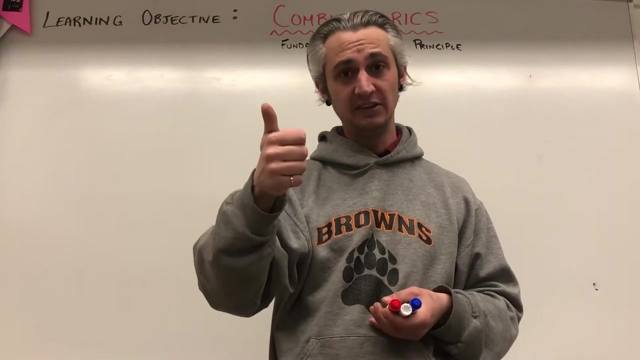 And combinatorics is essentially just the uh investigation of the different way we can arrange things. Um and combinatorics, the the big two, uh, the big two concepts in combinatorics are permutations where order of how we're how we're arranging things counts. 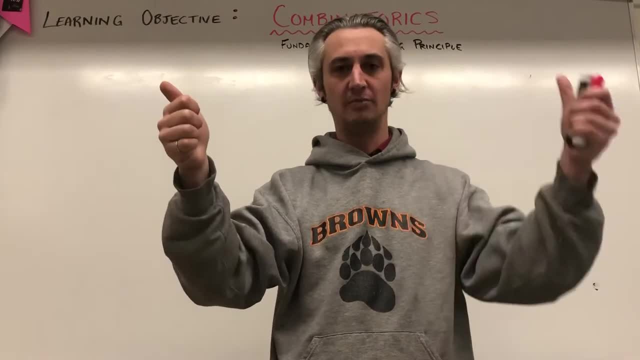 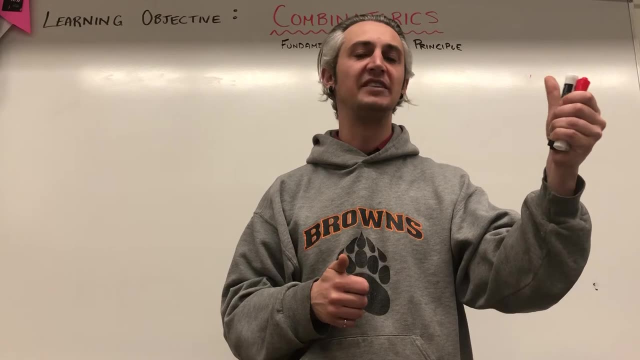 and combinations, or, uh, combinations. So permutations and combinations, Combinations. doesn't care about the order, Um, so it's like: how many ways can I select five? how many different ways can I select five letters from the alphabet right? 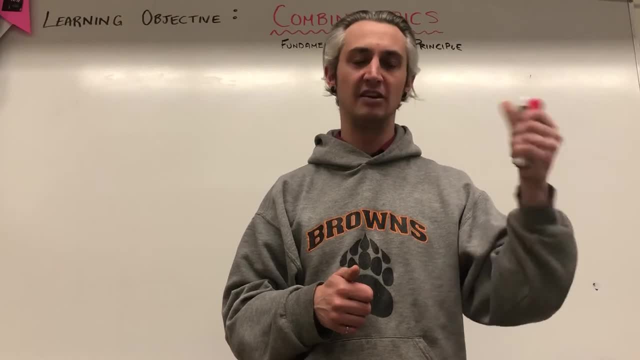 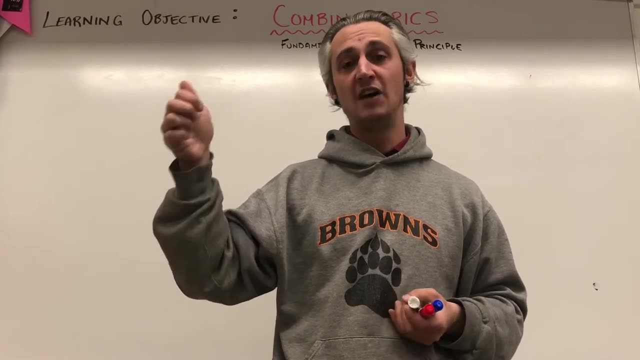 So it doesn't matter if you choose E first or if you choose E last, As long as you choose E and it's in there. that's a combination Permutations. however, would, if you're choosing five letters from the alphabet, 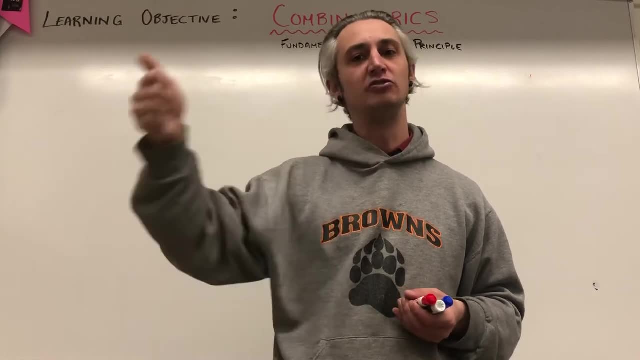 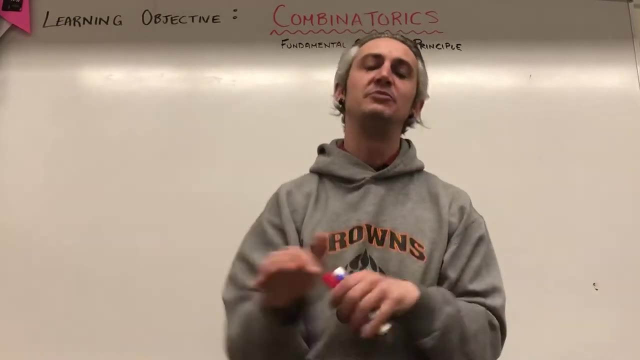 it would be concerned with: well, did you choose A first or did you choose A last? Because that's different, Whereas combinatorics would say: as long as I've chosen A, I've chosen A. But we'll talk about that more. I'm just kind of giving you a little sneak peek. 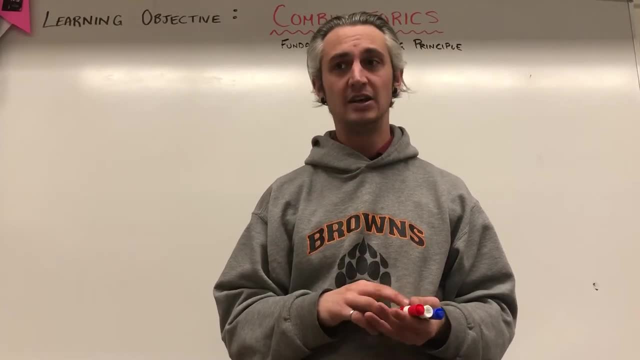 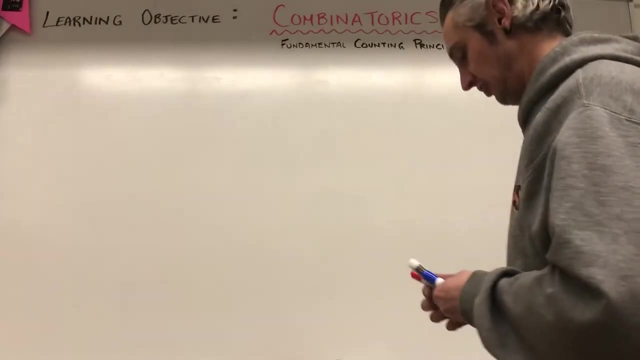 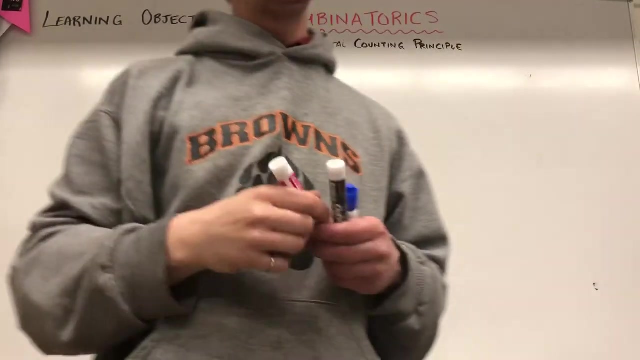 Um, but in order to work with combinatorics, uh, we need to first address just a couple kind of foundational concepts. okay, And those foundational concepts are related to the fundamental counting principle And essentially, the fundamental counting principle tells us that, if I can, um, 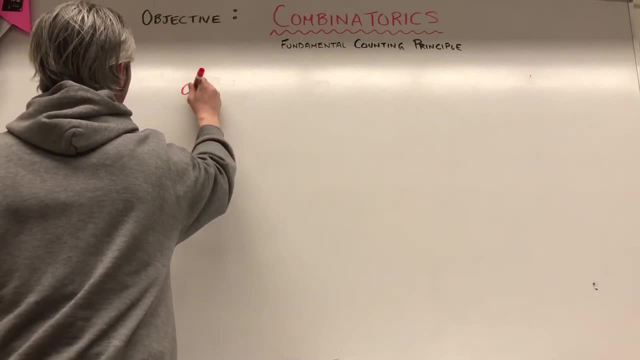 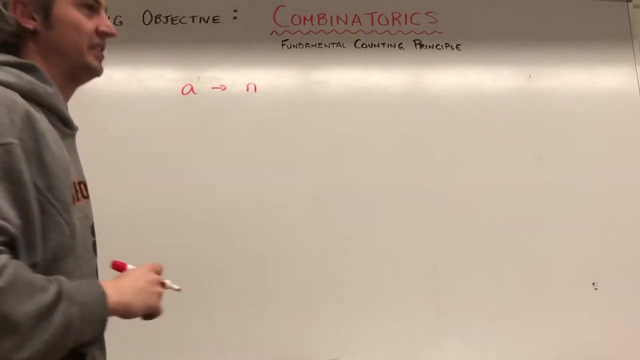 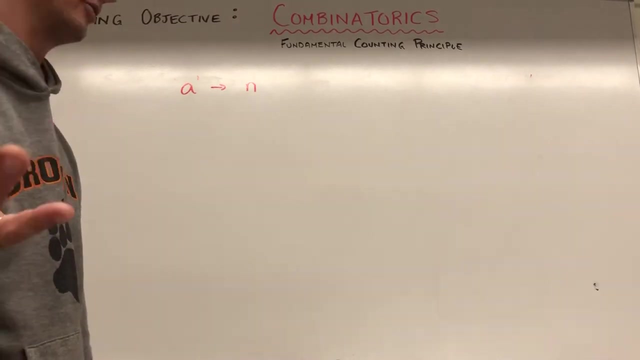 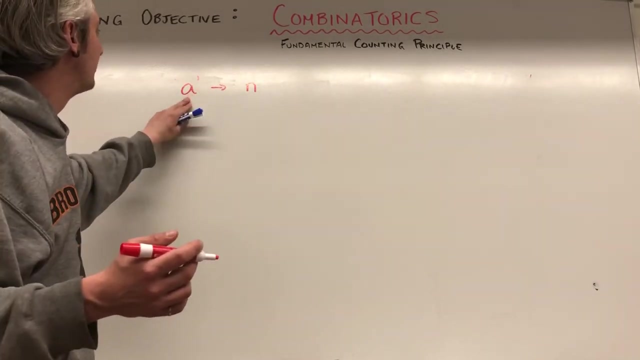 if I can do task A? um if I can do task A? n different ways, right. So say, how many ways can I? um choose a letter, letter from an alphabet? Well, 26 ways, right? So if I can do that, if I can do a certain, 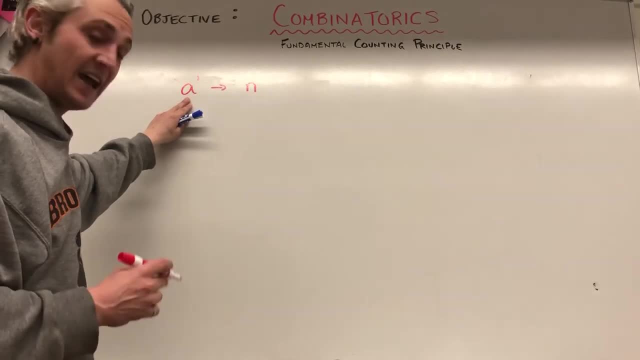 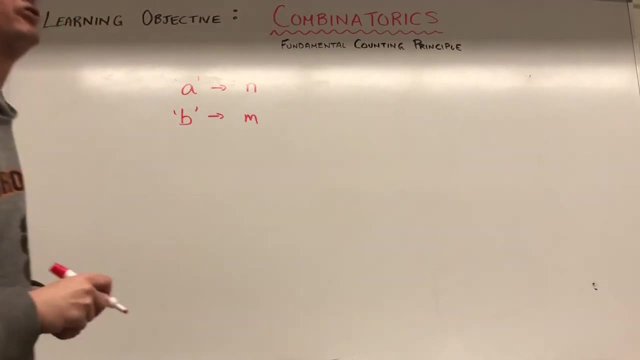 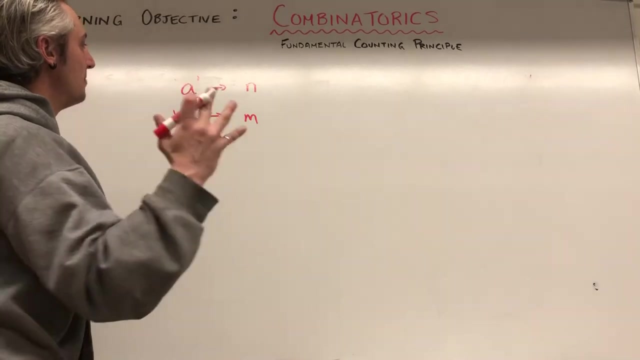 task that many ways and I can do a different task m ways. so say, how many ways can I choose a letter from the alphabet and how many ways can I choose a number from 1 to 10?? Well, the way that I can do, the total amount of ways that I can do this task and this task. 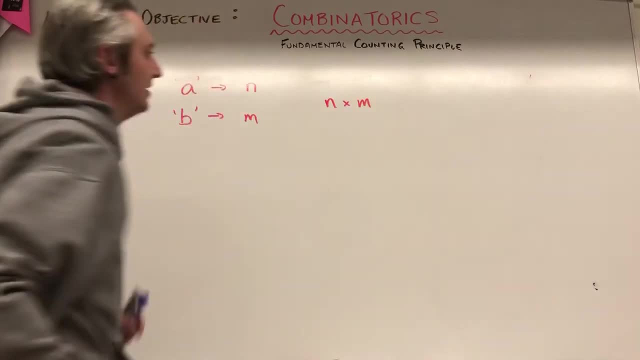 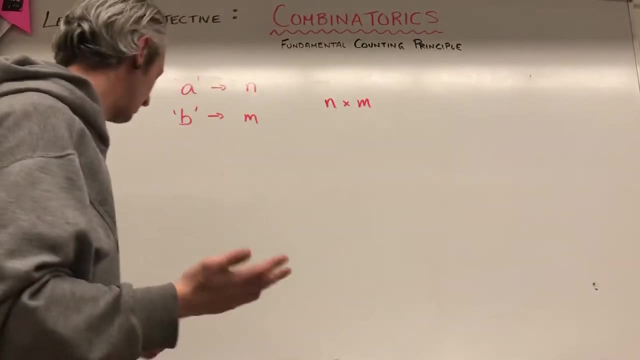 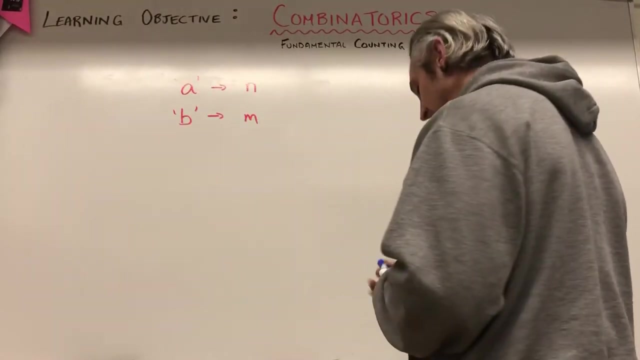 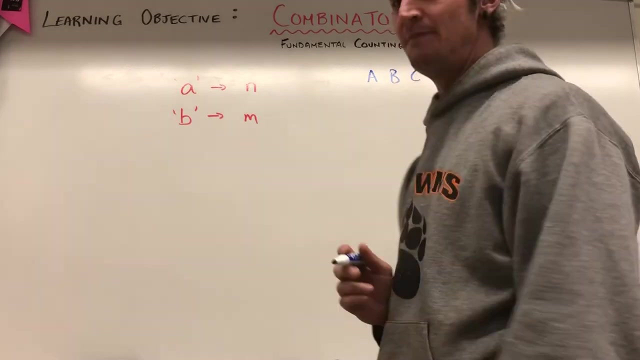 is simply n times m. okay, That is a fundamental counting principle. Now, what does that? I hope I explained that right, but let's look at it, okay. So what does that mean in practice? Well, let's say I have the letters a, b, c and we'll do d as well, okay, And I want to know how many ways. 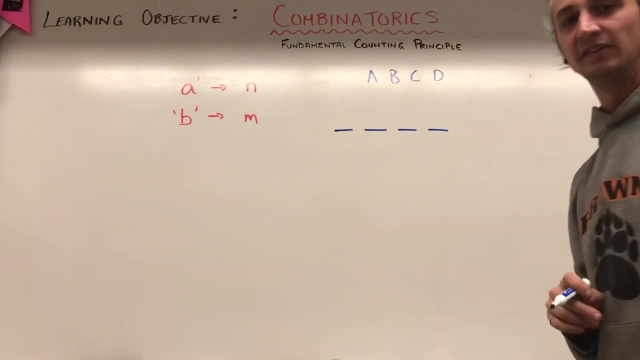 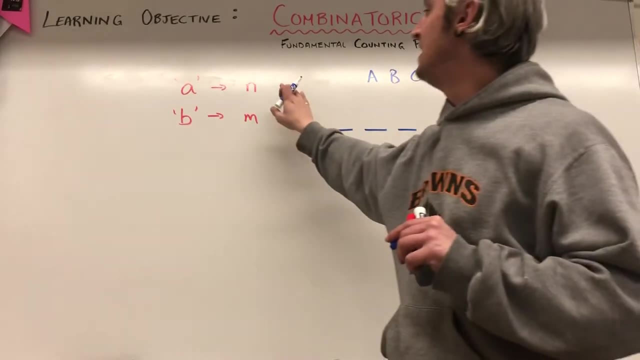 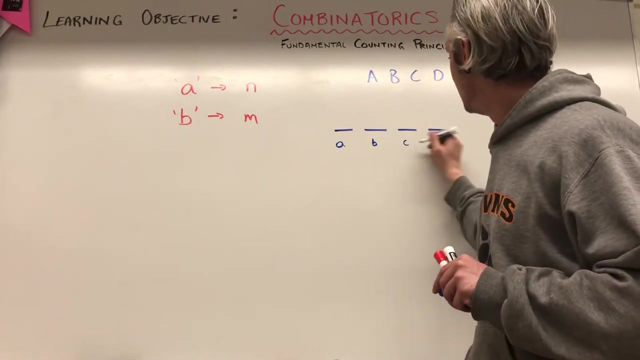 can I arrange those letters? How many different ways can I arrange those letters? Well, if we now have, this would be a, this would be b. I'm talking about task a, task b. this will be task c, task d. okay, 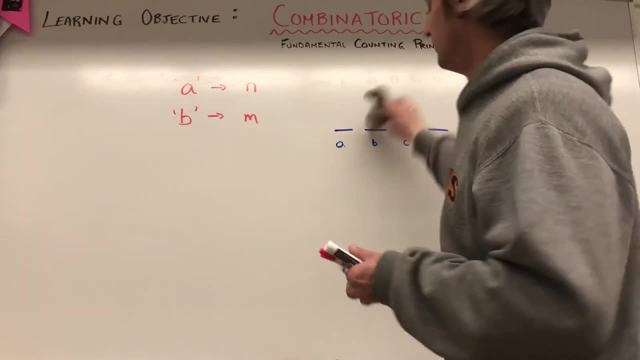 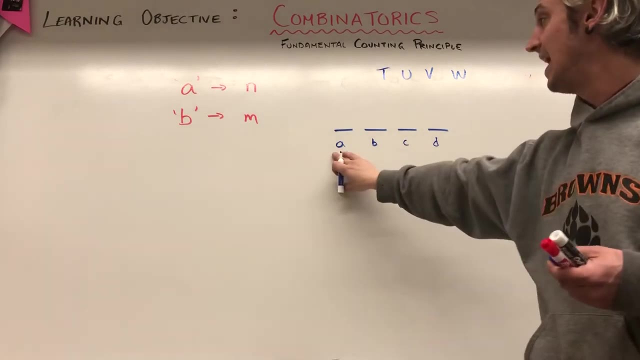 They're not. I'm going to use different letters just to so. let's say I had t u v w. How many ways could I okay? So this is my first task is choosing the first is choosing the first. 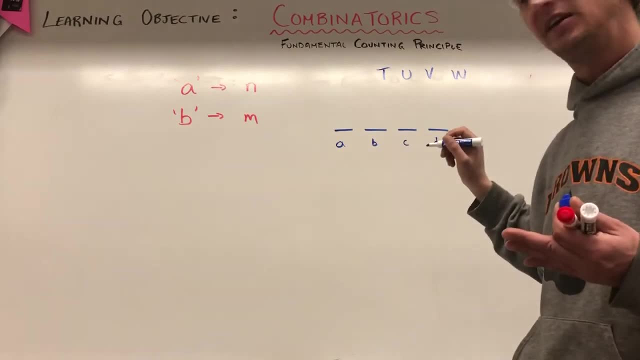 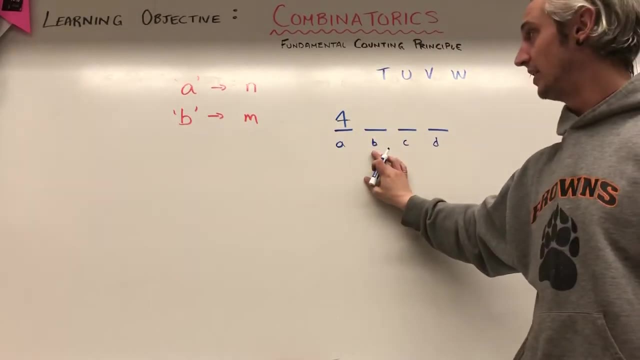 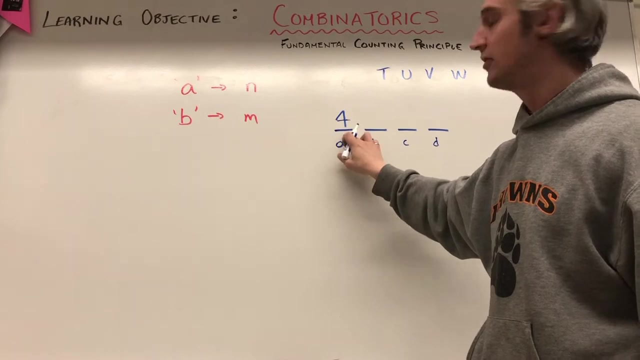 letter that's going to go in the first slot And I can do that. how many different ways I can do that? four different ways. right, I can choose four letters. The next task, we'll call that task b. how many letters am I like if I, if I put one letter here, one of the four goes here. 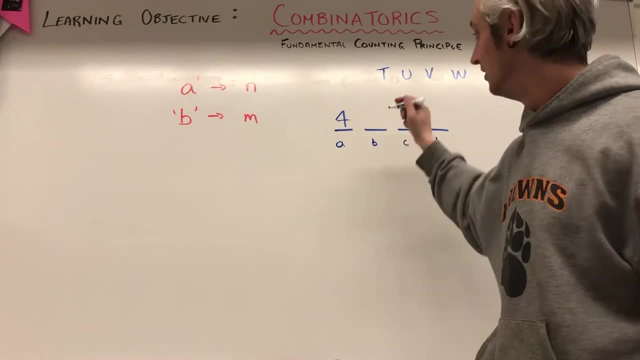 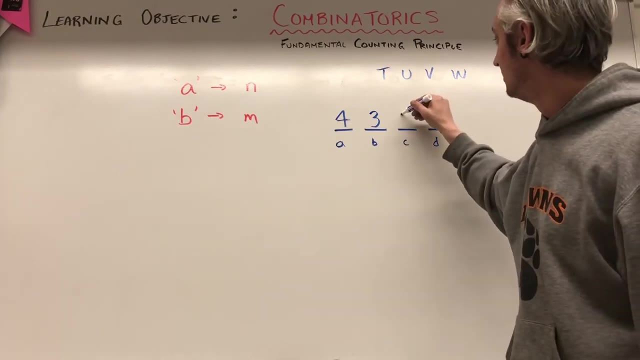 how many letters am I going to be allowed to choose from for the second task? It's going to be three. Now I have three to choose from. okay, C- there's only going to be two letters left. and d- there should only be one letter left And based on the fundamental counting principle to 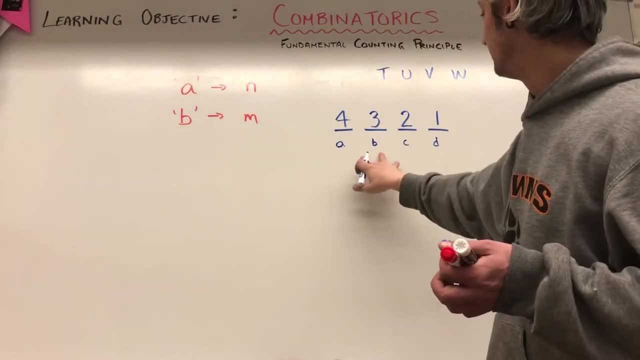 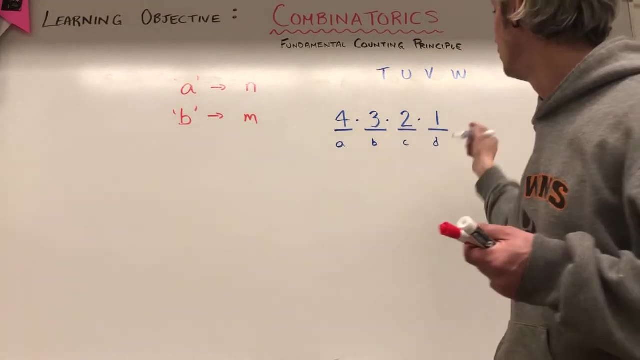 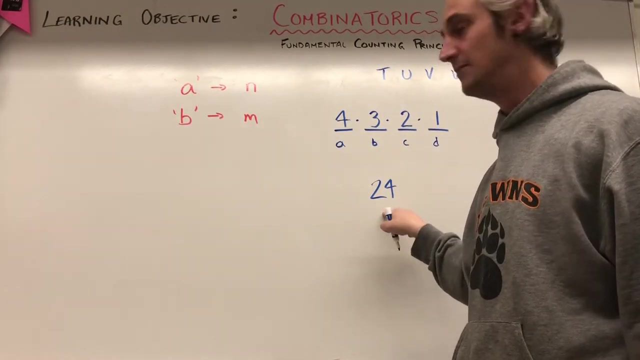 figure out all the total amount of ways that I can do this. this task is to multiply these together And I get: four times three is 12, times two is 24, times one is 24.. I can arrange the letters t, u, v, w 24 different unique ways And I got that from the fundamental counting principle. 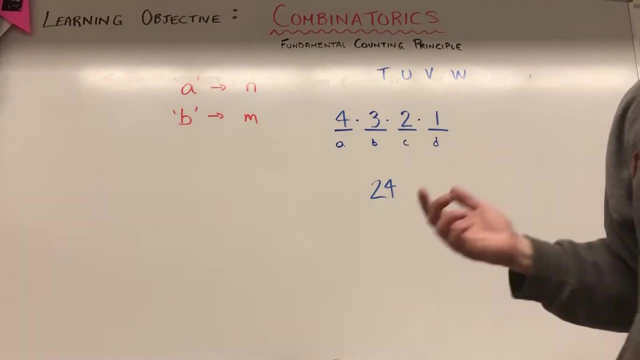 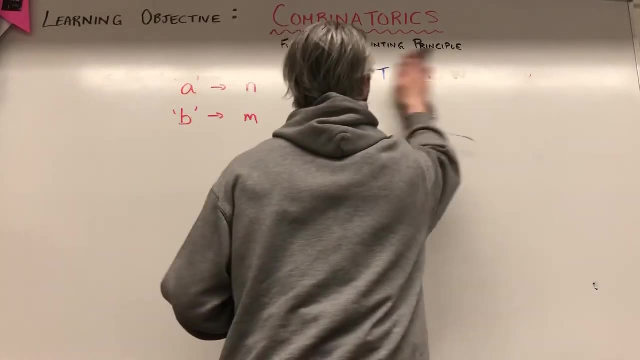 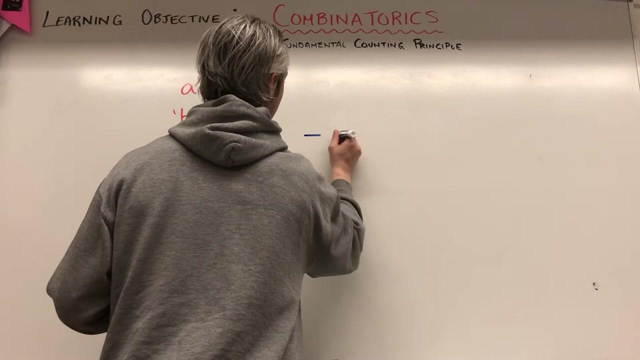 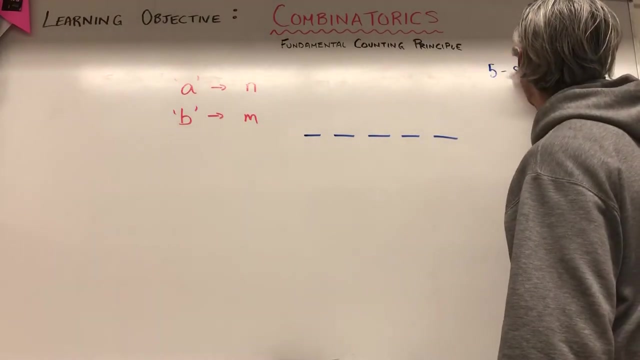 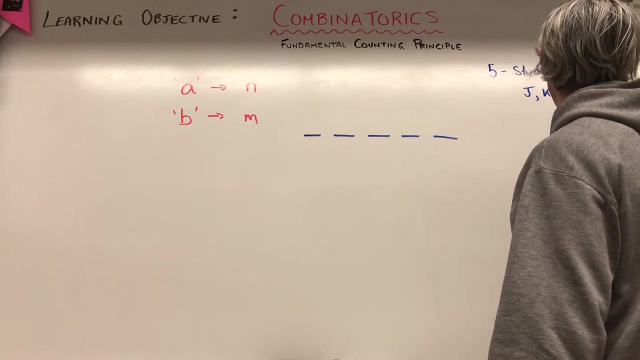 Um, let's see if, should I do it? example: yeah, so here's another example of that. let's say: I have, let's see, I have- five chairs. okay, I've got five chairs and I've got five students, five different students. so we'll call the students JJ as Jason翻, Jason K for. 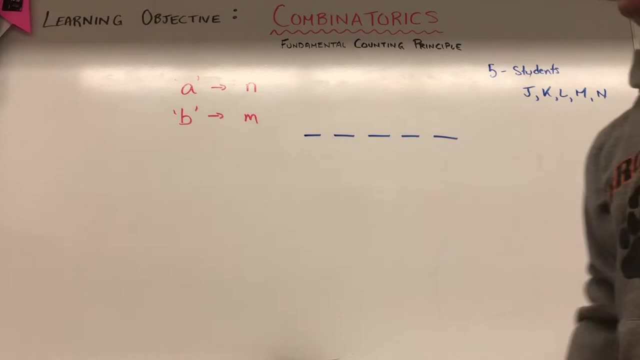 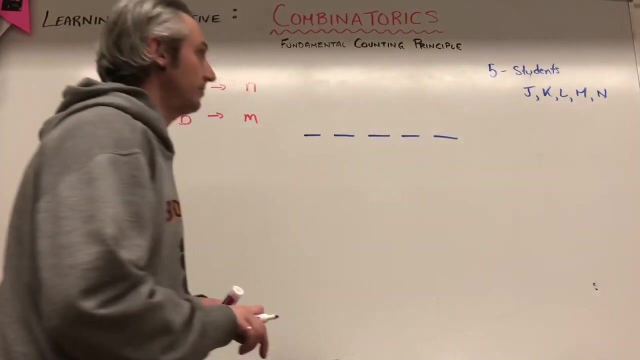 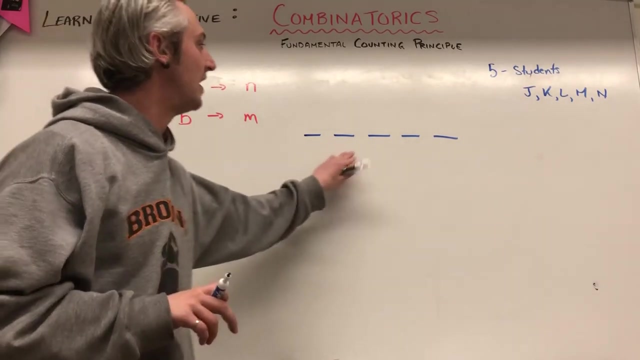 Caitlyn, alpha, Liam and format, and four and four, Nelson, woo, nelson. there we go. how many different ways can I arrange? how many different, unique ways can I arrange these students in the five chairs? now order matters, right. this is chair one. why one? you're? there'm three faculty of the five chair cast line. 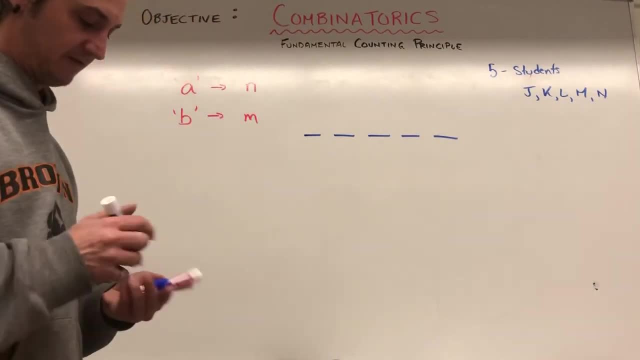 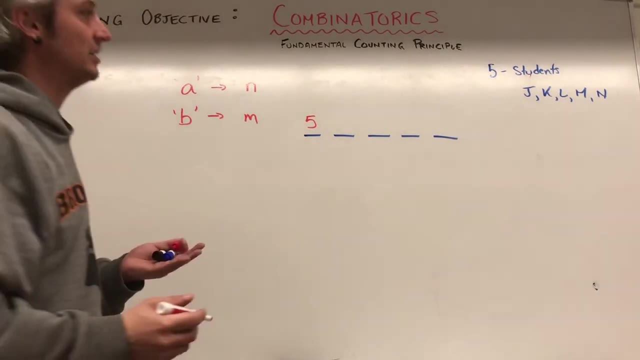 change. how many different ways can I arrange? how many different, unique ways. one chair two and chair three, chair four. Well, how many students can I pick from for the first chair? Five, Okay. How many students can I choose for the second chair? Well, I'm going to have lost. 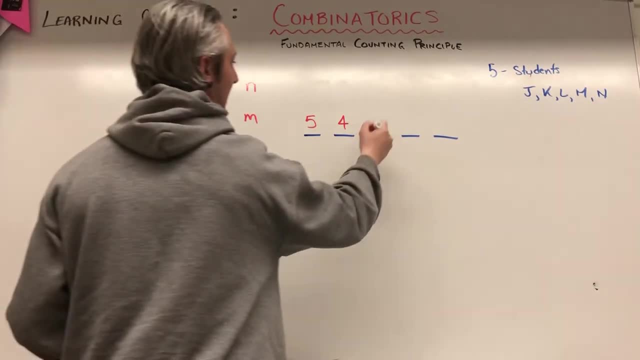 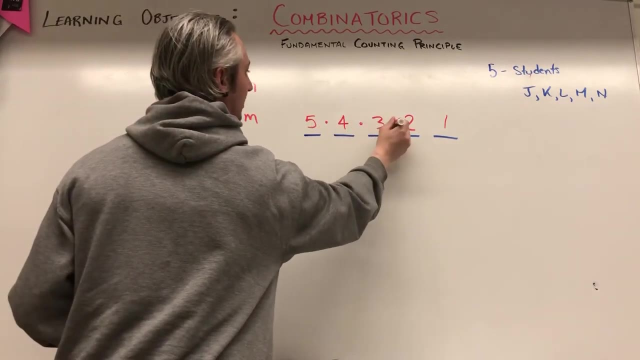 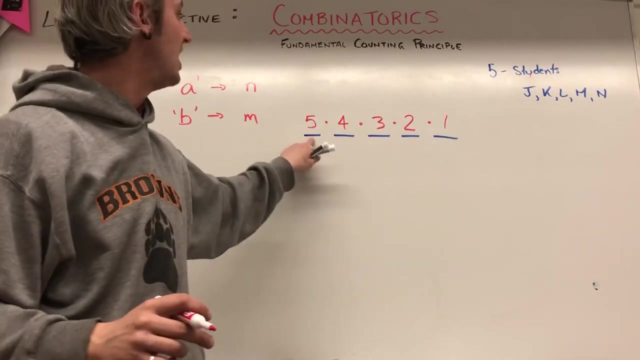 one student here, so it's going to be four, And then I'm going to have three students to choose from for the third seat, two left here and then one left there. And again, to figure out the number of different ways I can arrange these students in the chairs, I just have to multiply five. 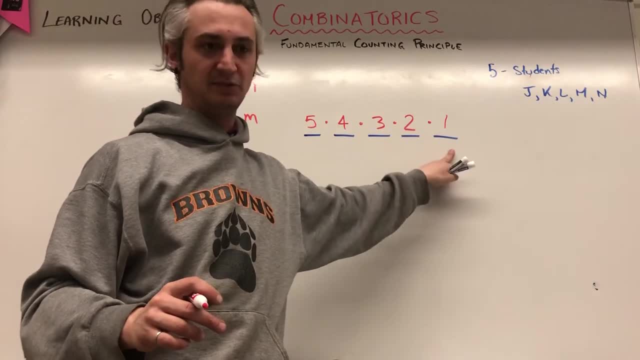 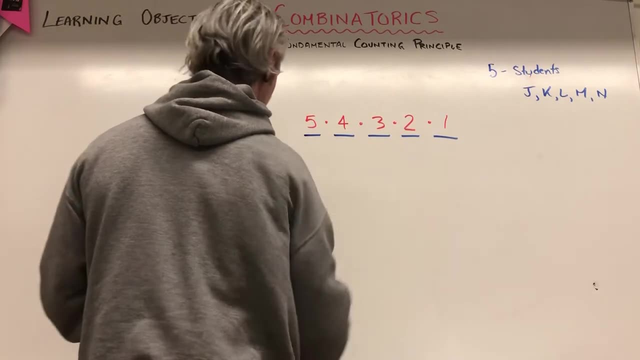 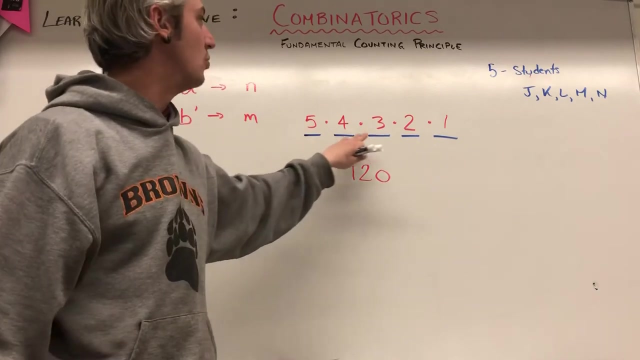 times, four times, three times, two times one, Okay, And in doing so I get to 20,, 60,, 120.. I can arrange these students in 120 unique ways, where seat one is right here and seat five is here. 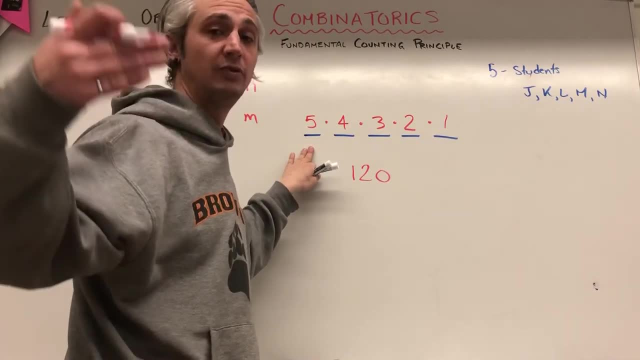 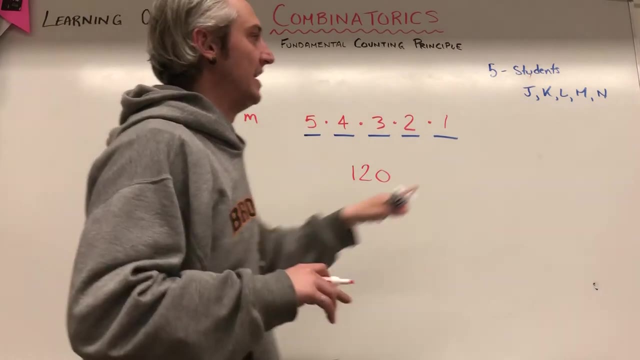 It's important that I keep track of the order. Now we're going to talk. When we get into combinations, the order doesn't really matter anymore, right So? but in this case there's only if this was a combination and order doesn't. 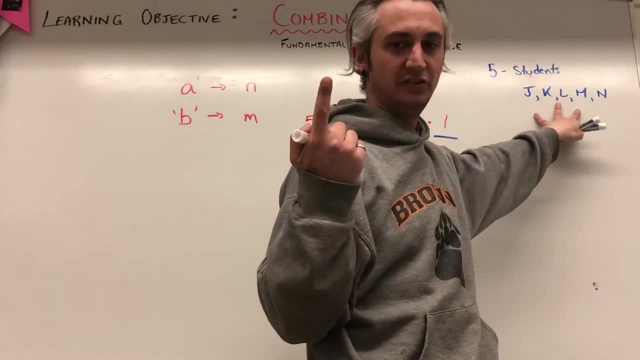 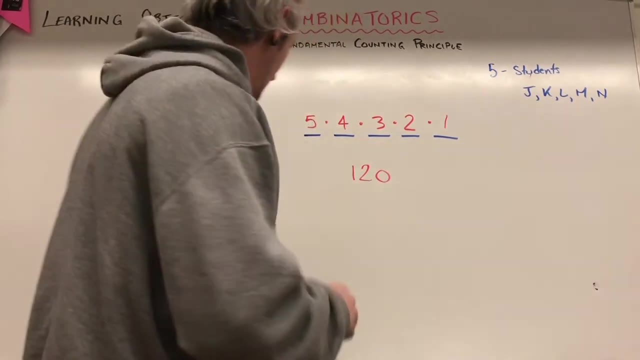 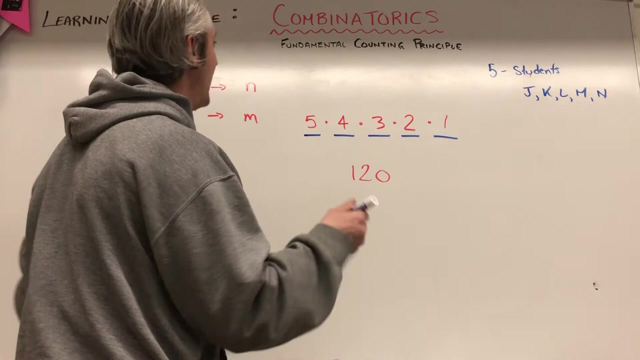 matter. there's only one way I can choose five students from the five students here. right, There's only one way, versus 120 when the order that I put them in matters. And so this leads us into the common, the mathematical concept of factorial Factorial. 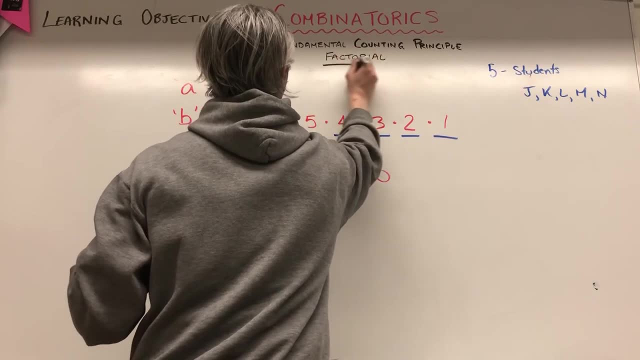 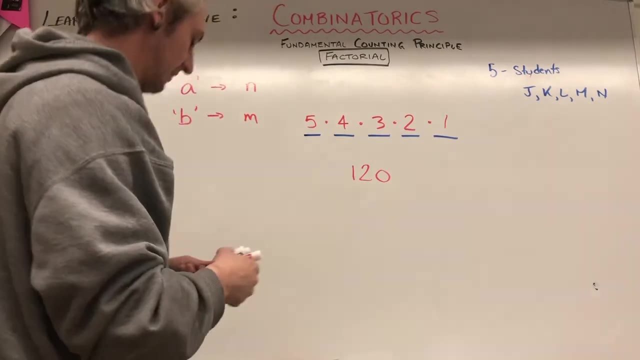 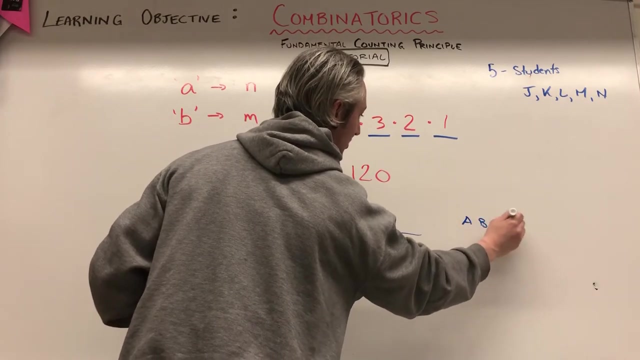 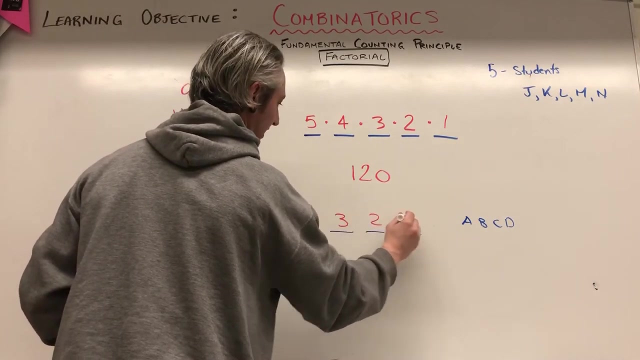 Okay, In fact, Foyle just says: when I get into a situation like this or a situation like the last one where I was, where I was arranging the letters A, B, C and D into unique combinations for order matters, And this one I had four times, three times, two times one, Okay, I can rewrite this as: 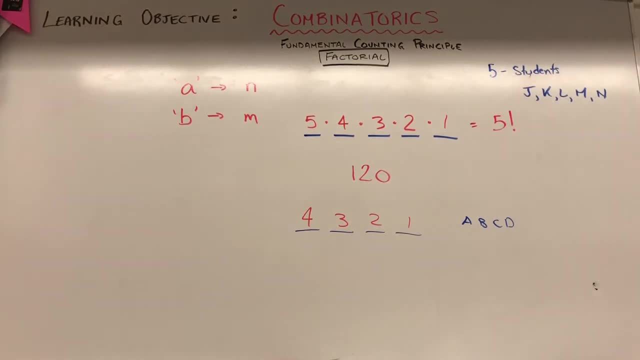 I can rewrite this as 4 factorial. What does 5 factorial mean? 5 factorial just means 5 times 4 times 3 times 2 times 1.. 4 factorial just means 4 times 3 times 2 times 1.. 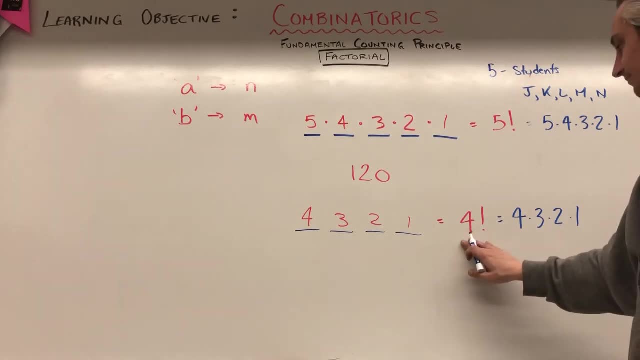 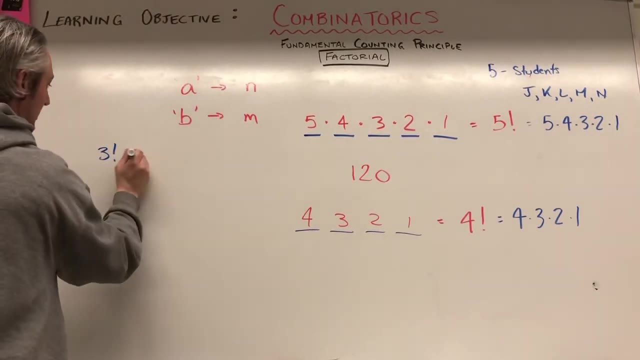 Basically all the numbers leading up to that number we multiply together. So what would 3 factorial be? It would be 3 times 2 times 1.. What would 8 factorial be? It would be 8 times 7 times 6 times 5 times 4 times 3 times 2 times 1.. 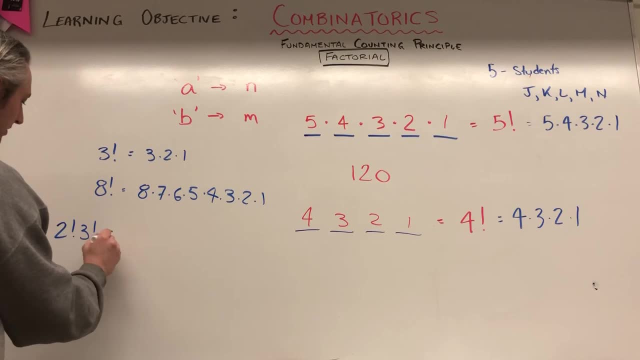 What would 2 factorial- 3 factorial be? Well, it would be 2 times 1 times 3 times 2 times 1.. What would 4 factorial 3 factorial be? Well, it would be 2 times 1 times 3 times 2 times 1.. 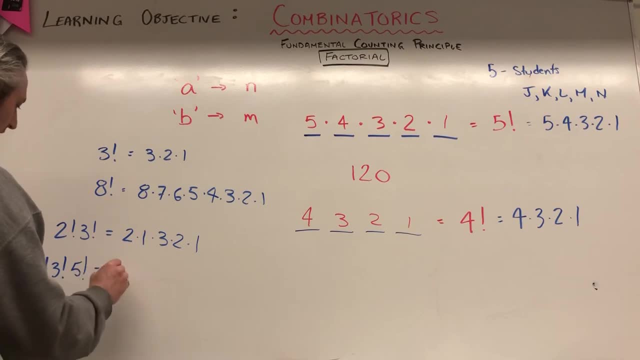 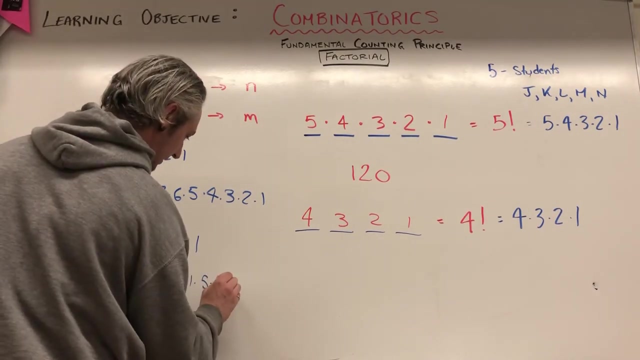 3. factorial 5. factorial b: Well, it would be 4 times 3 times 2 times, 1 times, 3 times 2 times 1 times 5 times 4 times. What the heck is that Times 4 times 3 times 2 times 1.. 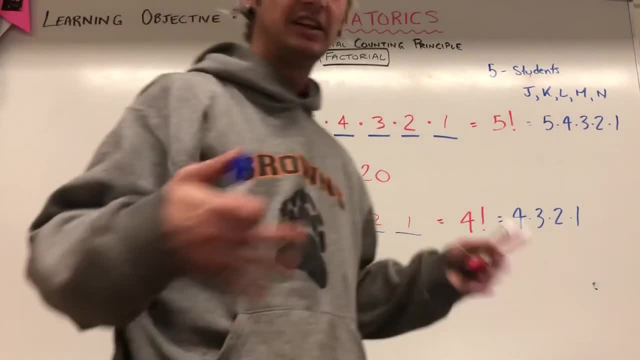 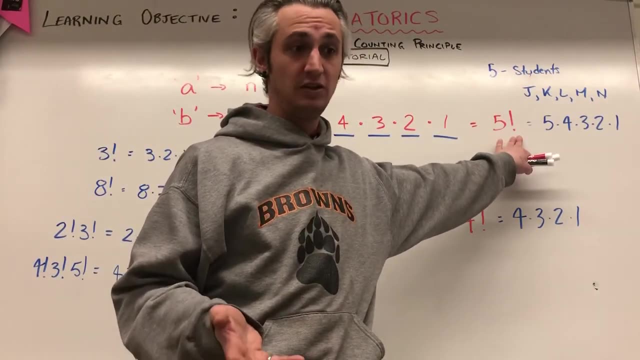 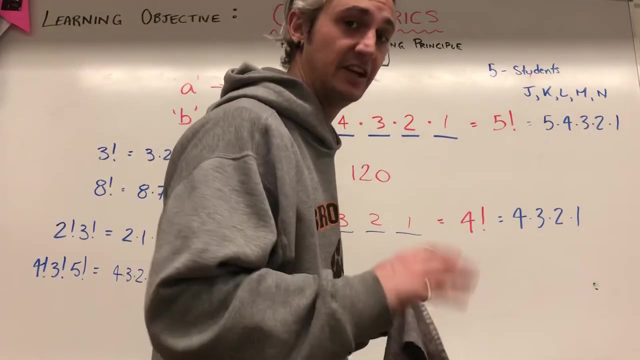 Big number. That is factorial. It's a new operational sign, Just like multiplication, division, and factorial is a mathematical symbol that we use quite often. So those are the fundamentals. That's what we just need to kind of acknowledge is the fundamental counting principle here. 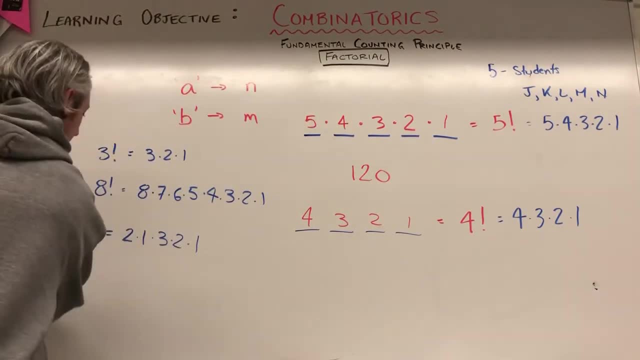 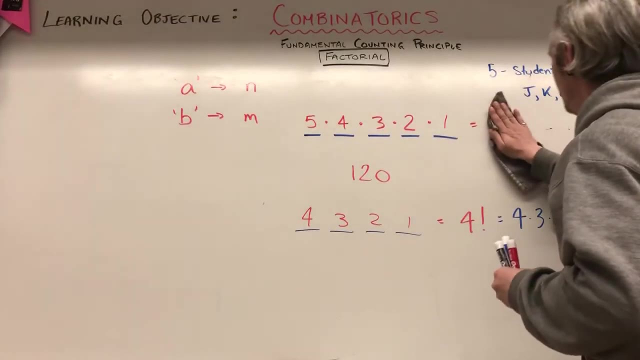 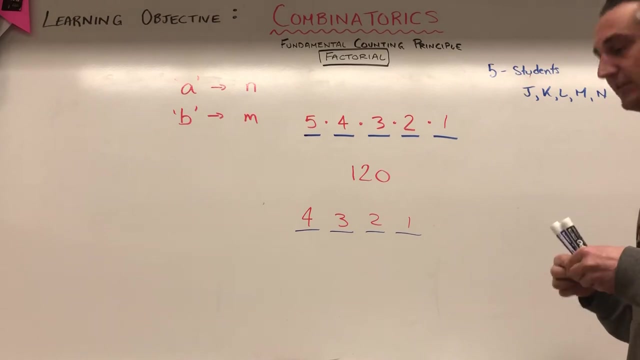 and factorial, which is shorthand. Now, in these examples that I did here, there were a couple assumptions I made right. The first is that there was, They weren't assumptions. My examples just didn't include certain things. The first was repetitions. 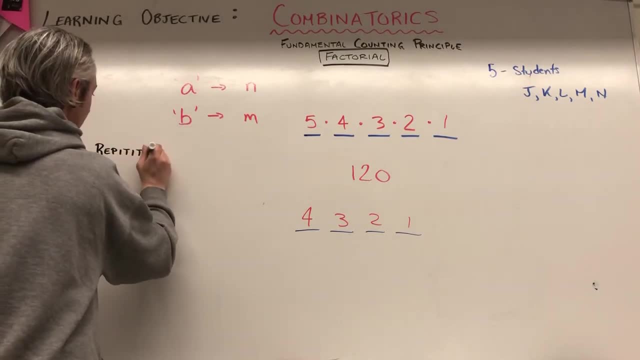 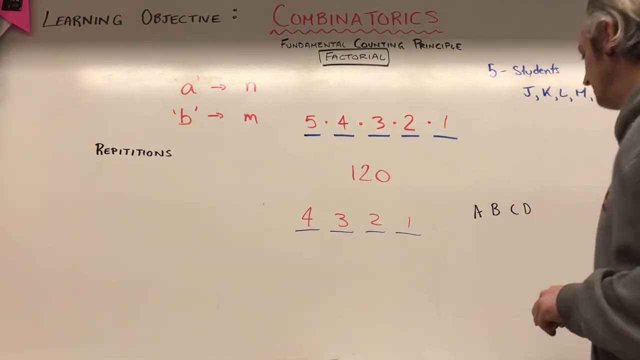 Okay, I had no repetitions here When I chose A, B, C, D. that's different than if I would have said: how can you arrange the letters A, A, C and D? Okay, A is the same. 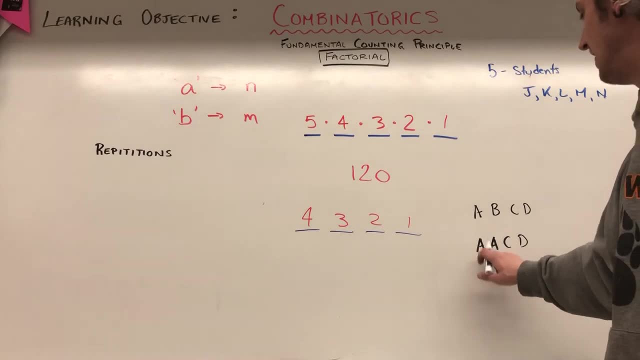 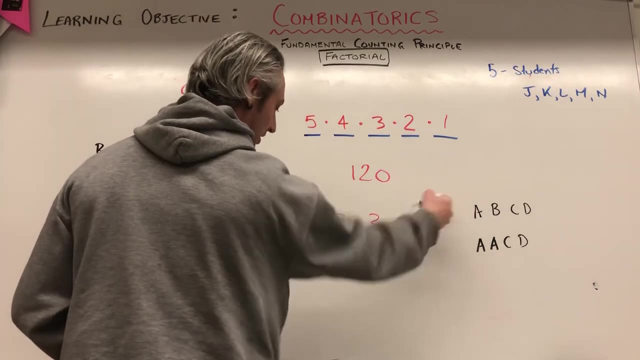 A is the same as A, So these two are repeated and that creates a different case. And in essence what happens in that case is it becomes 4 factorial, just like over here, but then I divide by 2 factorial for my repetitions. 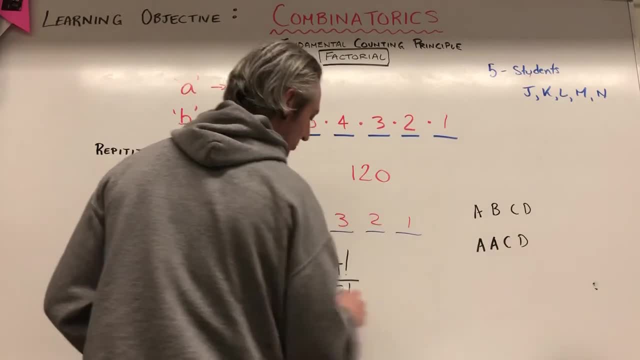 I have 2 repetitions, 2 factorial. If I had A, A, A, D, it would be 3 factorial down here. So we'll talk about that in the next video. And then the other thing we didn't talk about: 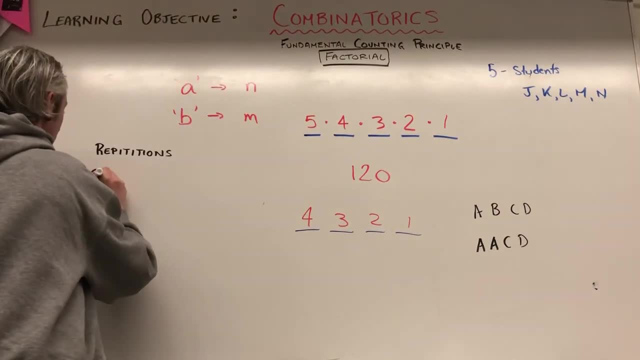 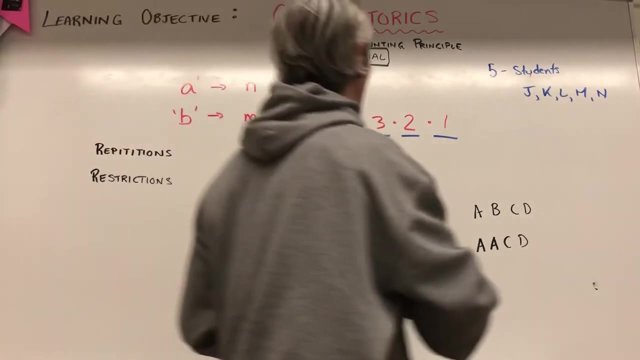 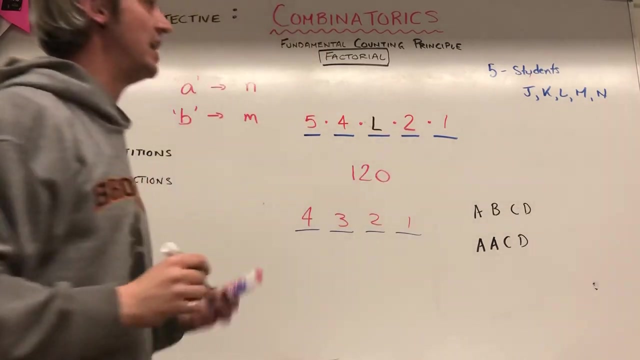 is restrictions, Okay, When I give you certain restrictions on what you can do. so an example for that up here was: how many ways can I arrange these students if the third chair always has to be student L? There's a restriction And in this case it would be. 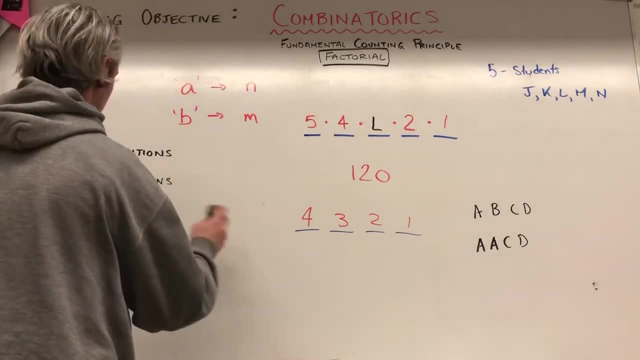 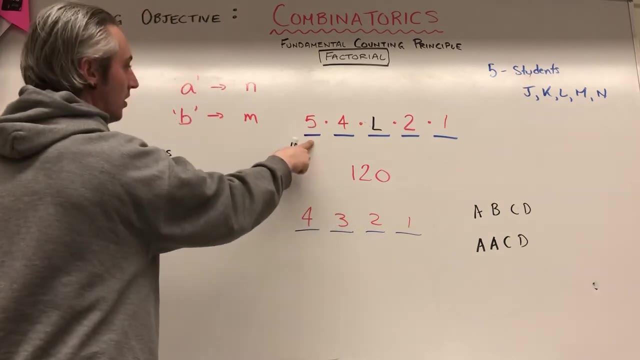 well, it would be 4 factorial times 3 factorial. No, it would be 4 factorial. No, sorry, It would be 4 times 3 times 1.. It would be 4 times 3 times 2 times 1.. 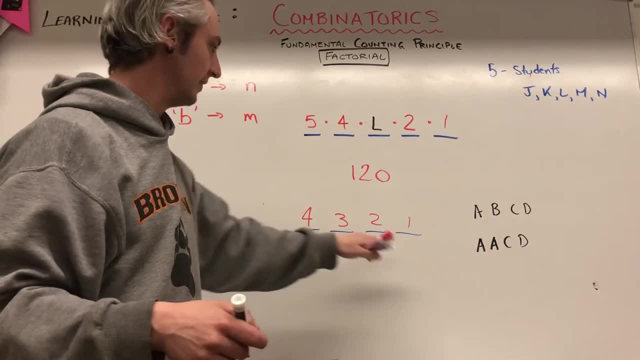 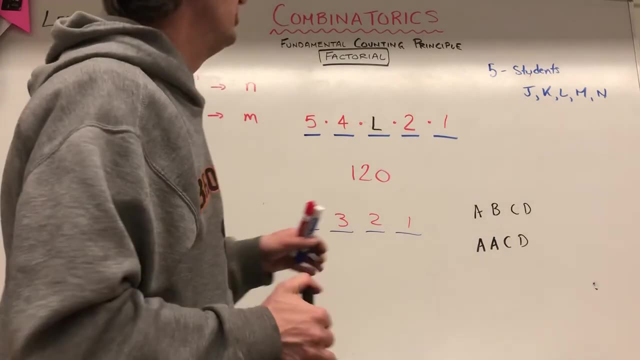 There wouldn't actually be a formula for this one, like there was down here, But in the next video we'll talk about all of that. At this point, you just need to know that when we are arranging unique, when we are arranging items, 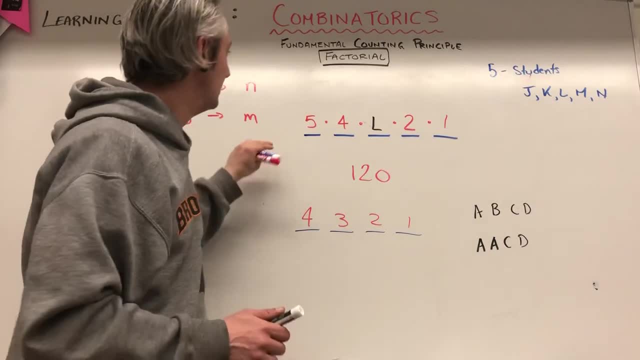 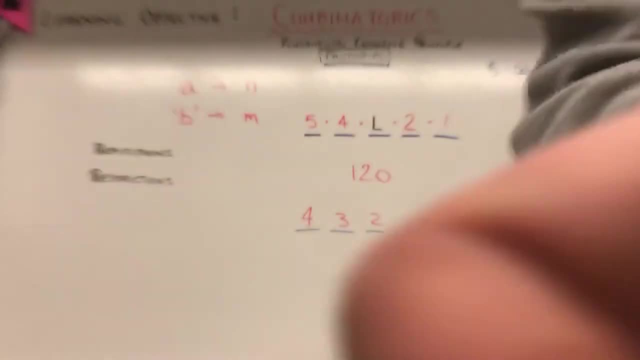 that there's no repetitions and no restrictions. we can just basically use the amount of items that are factorial, And that will tell us how many ways we can arrange them. So thank you so much for watching And I'll see you in the next video. Bye-bye.